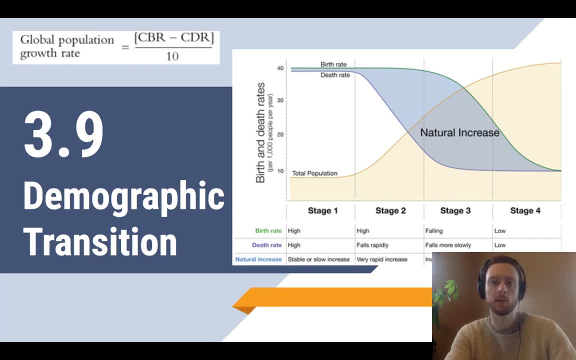 to basically have zero growth. So in phase two the country becomes more developed, so it has more access to clean water and health care. This causes death rate to decrease, but birth rate remains high, so the population grows. Then in phase three the birth rate begins to fall as family income and 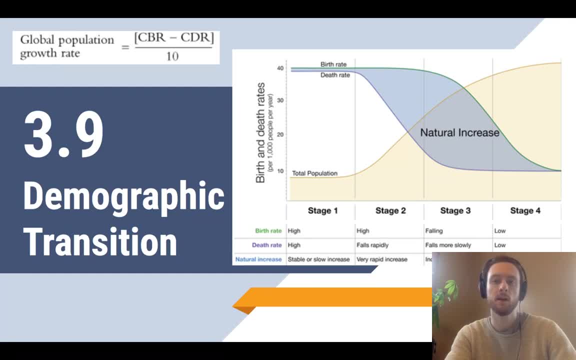 educational and economic opportunities for women increase. Population is still growing, but the rate of growth slows quite a bit as birth rate comes closer to death rate. Then, finally, in stage four, both birth rate and death rate are quite low, so the population growth slows to close to zero. 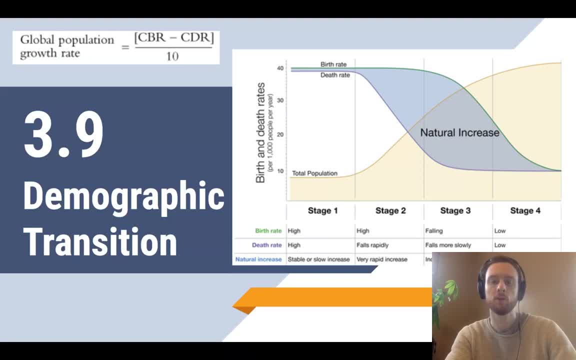 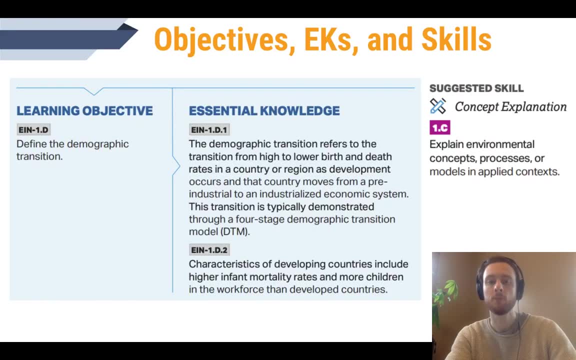 and may even begin to decline. We'll talk more about the different indicators of these phases and what they mean for a country's development throughout this video. Our objective for today is to be able to explain the process of demographic transition. In order to do that, we need to understand what development from a pre-industrial to 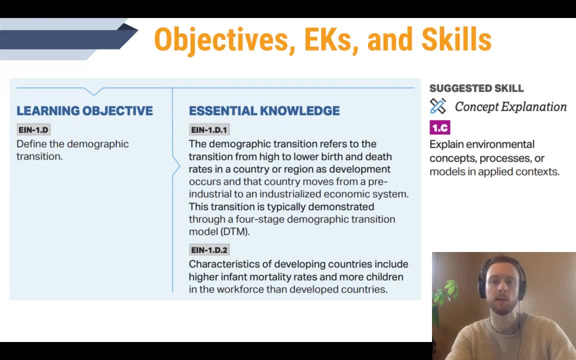 an industrial economy looks like and what it means for the birth rate and death rate of a country. We also need to understand that developing or pre-industrialized nations usually have higher infant mortality rates, as well as more children in the workforce, primarily in agricultural farm work that provides the family with income. 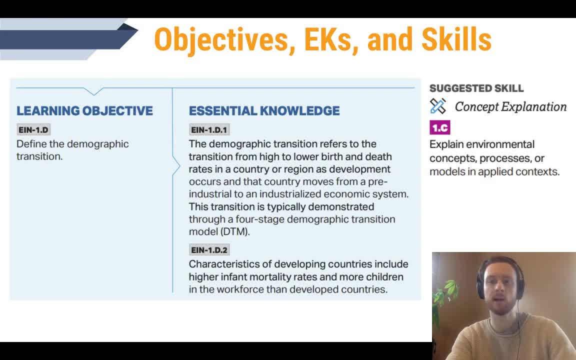 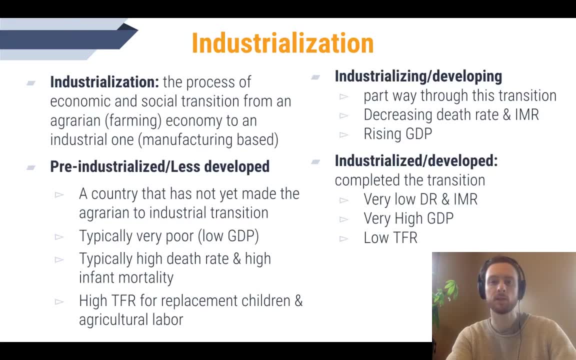 And then our science practice for today is explaining environmental concepts, processes and models in an applied context. So before we talk about the actual steps of demographic transition, we need to go over what industrialization is. So it's the process of a country transitioning its social and economic systems from an agrarian based society to an industrial society. That means 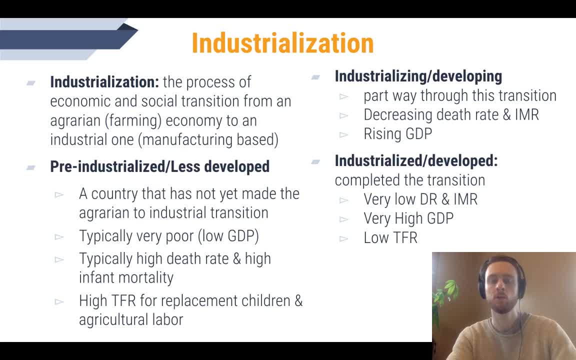 one based on farming for food and for income to one that's based more on manufacturing of goods and providing of services for income. So pre-industrialized nations, sometimes referred to as least developed nations, have not really started the transition of industrialization yet. They're typically very poor nations where citizens have very low incomes and often grow their own. 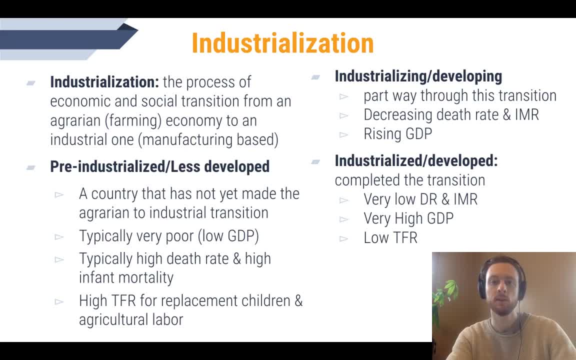 food and earn their income by selling excess food. Since access to clean water and health care is low, infant mortality rate and death rate are very high in these countries. TFR is also high due to factors: lack of educational opportunities for women, the need for replacement children and also the need 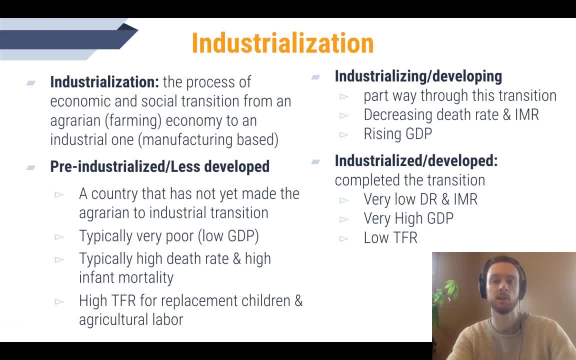 for children to provide this agricultural labor that we mentioned earlier here. Then we have countries that have begun industrializing, and we often refer to these as developing nations. They have decreasing death rates and infant mortality rates, increasing GDP, but there are still portions of their population that are living in agrarian 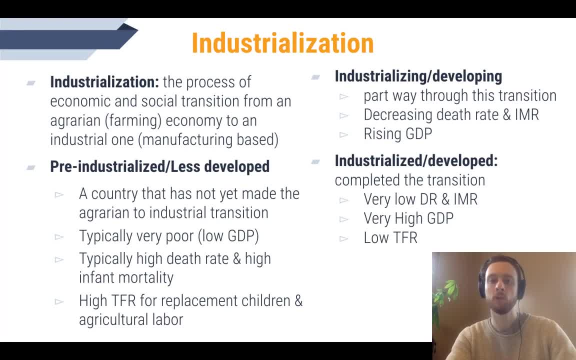 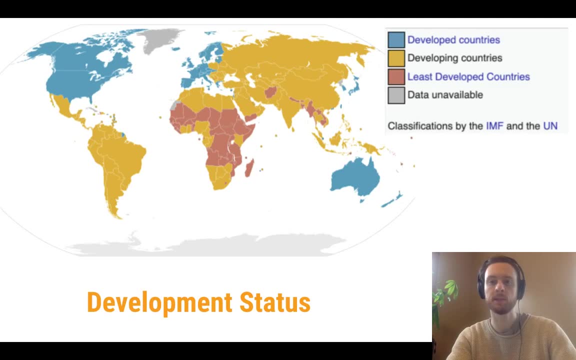 societies And finally, we have fully industrialized or developed nations. These are ones who've completed this transition and they have low death rate and infant mortality rates, very high per capita GDP and very low TFR. This map of the world here can help us get a better. 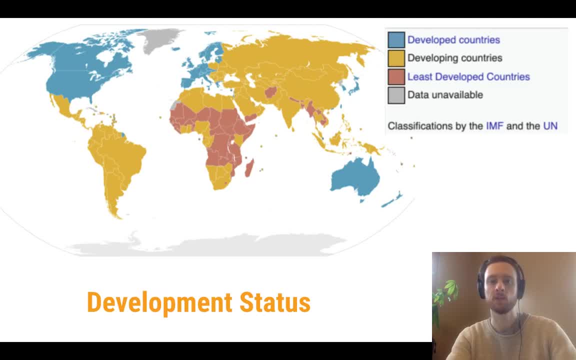 sense for the development status of different countries, And so we can see in blue. we have the US, Canada, Australia, most of Eastern Europe. These are all what we would consider developed nations. So they've completed the transition from agrarian society to industrialized society. 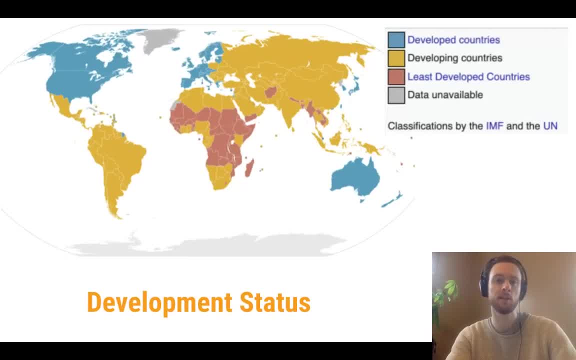 If we look at the yellow, though, we'll see that most of the world is actually in the developing stage, meaning that many parts of these countries have transitioned to more wealthy manufacturing and service-based economies, but portions of these populations are still living in agrarian societies. 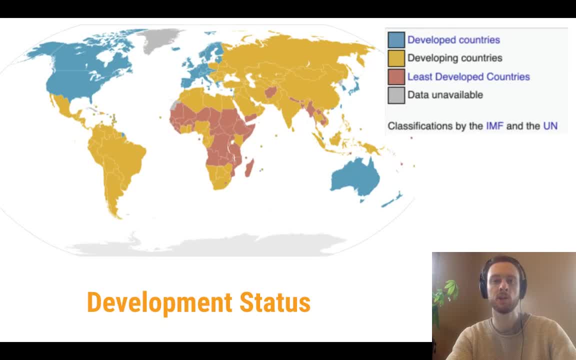 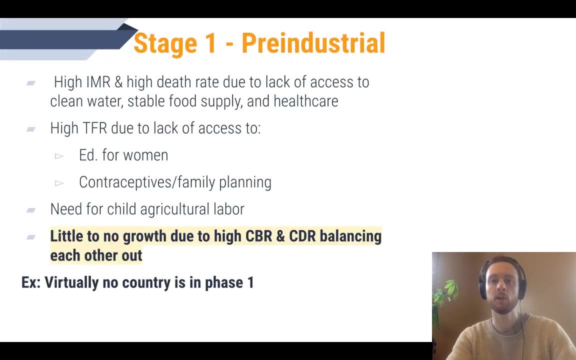 And then, finally, we have much of Africa and portions of Southeast Asia that are considered least developed or early in their industrialization, And this means that the majority of their residents are still living in agrarian economies and have not yet made the leap to the next level of industrialization. Now we'll talk about the four stages of demographic. 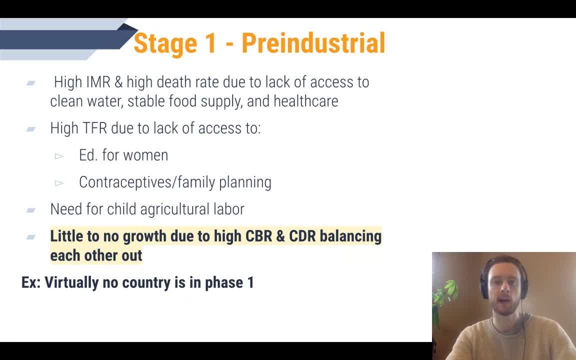 transition starting with phase one or stage one. In stage one, a country has a high infant mortality and death rate, and this is due to lack of access to clean water, stable food supply and health care such as hospitals and vaccines. TFR is also high due to lack of access to educational opportunities. 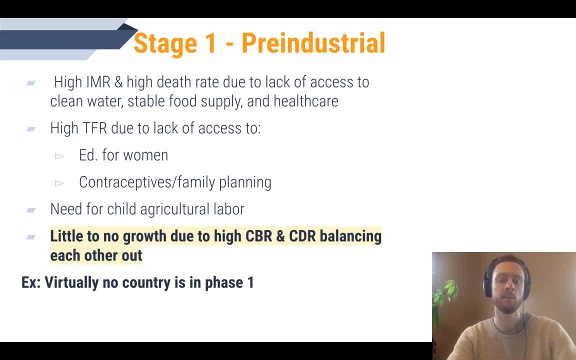 for women- access to family planning and contraceptives, and then that need that we discussed earlier for child labor terms, This means that many countries are still in the pre-industrial stage and they have the ability to provide income for the family, Because CDR and CBR are both so high. 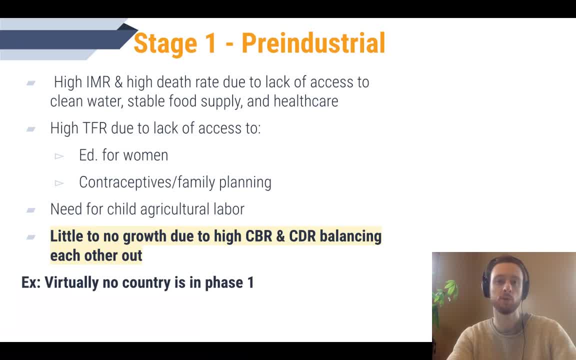 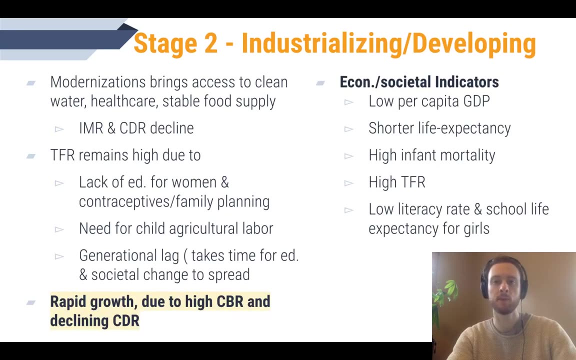 the country has a stable population without much growth. It's important to point out, though, that there are virtually no countries in the world that are still pre-industrial, so, while many nations are very poor and are very early in their development, essentially every country has moved from stage one into stage two and is growing to some degree. 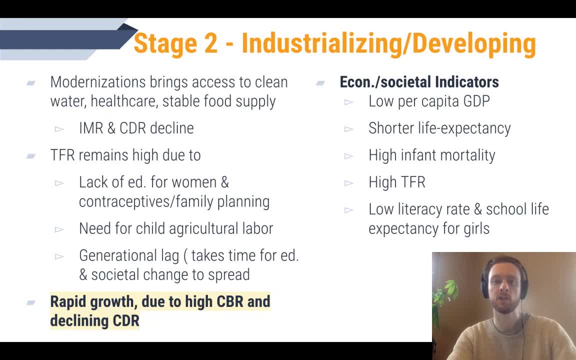 Next we have stage two, which is where most of the world's population is currently. Stage two: modernization has begun and parts of the country are making that shift from an agrarian economy to a manufacturing-based one. This brings increased wealth and access to clean water, a more stable food supply, healthcare. 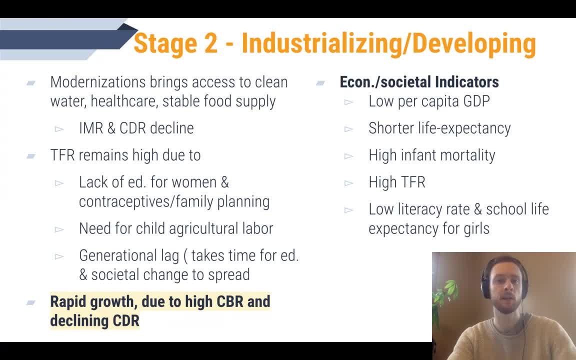 access for more people. so more children are surviving, they're getting vaccines, they're getting the nutrition they need, so we're going to see infant mortality rate and death rate drop pretty substantially. However, TFR remains high, since educational opportunities for women often still lag behind. 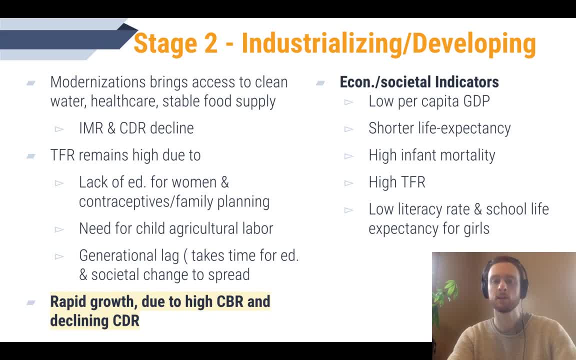 men, and access to contraceptives and family planning are slow to become available. There's also the need for parts of the country to still rely on agriculture for their own food needs and their income, which is going to cause them to have more children to provide. 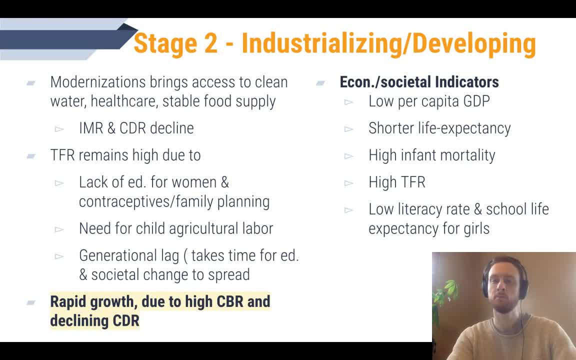 that labor and that income that they need. And then there's an important concept called population momentum or this idea that there's kind of a generational lag. It takes a long time, meaning it takes a long time for culture and societal norms of having 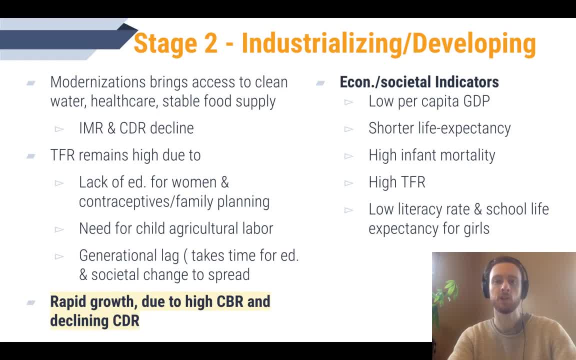 a lot of children to shift, So it takes a long time for the changes brought on by education and increased income to make their way throughout a population. So the TFR remains high for about a generation, which could be decades, And so TFR is going to remain high through much of stage two. 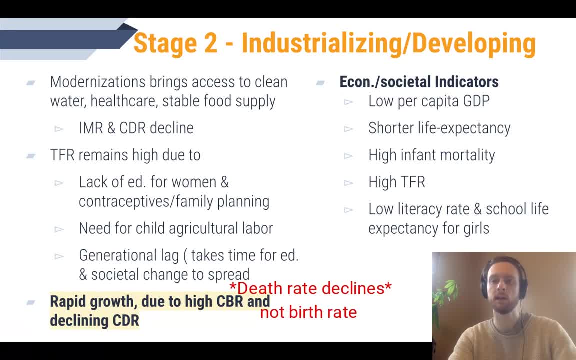 Because TFR remains high but birth rate has declined. these countries experience rapid population growth. These are countries like India, Brazil, China, Afghanistan And then, if we look over at the right, we have some indicators of stage two countries. So, even though they've started their development, they're typically going to have lower per capita. 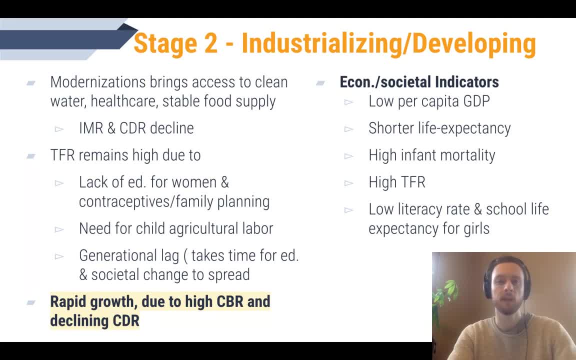 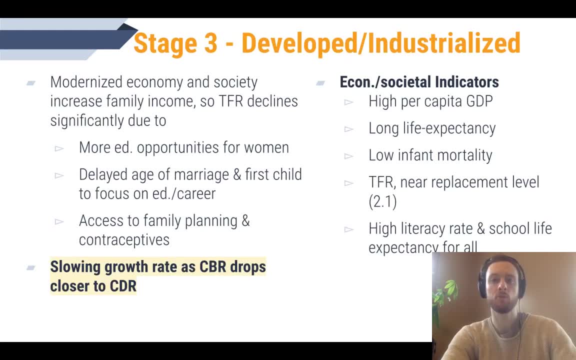 GDP or lower per person wealth, And they're also going to have lower literacy rates and lower educational opportunities for women. Next, we have stage three countries which we would consider developed nations. In these countries, modernization has increased family income substantially, Decreasing the need for children to provide labor and income. 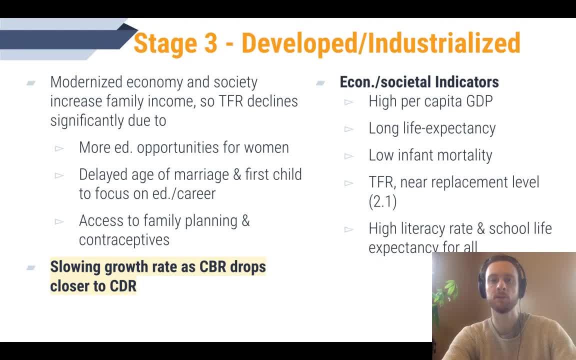 TFR also declines due to increased education opportunities for women, delayed age of marriage and first child for both men and women as they spend more time pursuing education and careers, and access to family planning and contraceptives become far more widely available. In stage three, growth slows down as the CBR drops closer to the CDR. 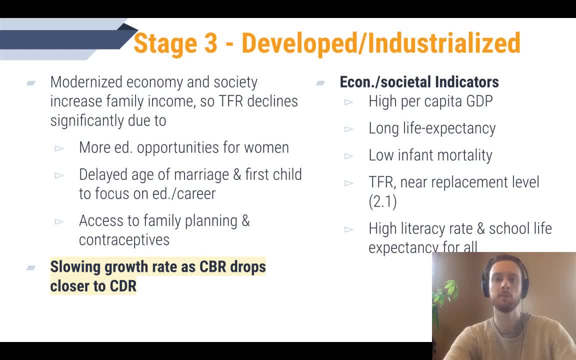 So birth rate moves closer to death rate. So these countries will typically have- We have a TFR that's closer to replacement level of 2.1.. They have low, stable growth that is slowing down, getting closer to zero growth. They also have very high per capita GDP, long life expectancy and other indicators of affluence. 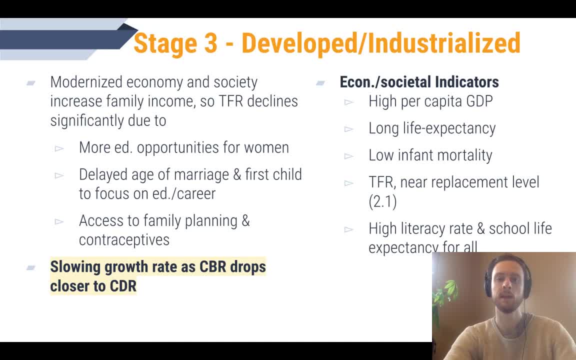 such as long educational lifespan for women and just an overall higher standard of living. If we want some examples here, we have the United States, Canada and much of Europe. And finally, we have the United States, Canada and much of Europe. 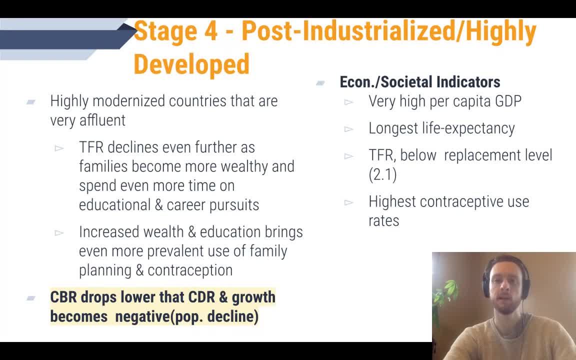 And finally we have stage four: countries that have become so affluent that TFR has actually declined below replacement level. fertility and their populations have started to decline So as economies become highly modernized and family income rises further, families are just having far fewer children. 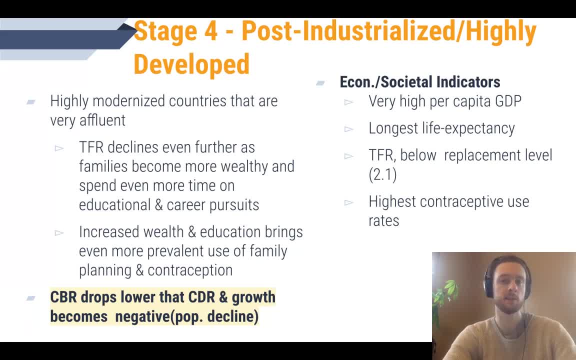 They're spending more time pursuing educational and career opportunities and this leaves less time for raising a family and also delays the age of marriage and the age of first child, And all of these factors lead to To a lower TFR. If we want to look at indicators of a stage four country, they would have the highest. per capita GDPs in the world. typically They're also going to have very high life expectancy, meaning that a large portion of their population is elderly, And they're also going to have TFR that is below replacement level, so below 2.1.. 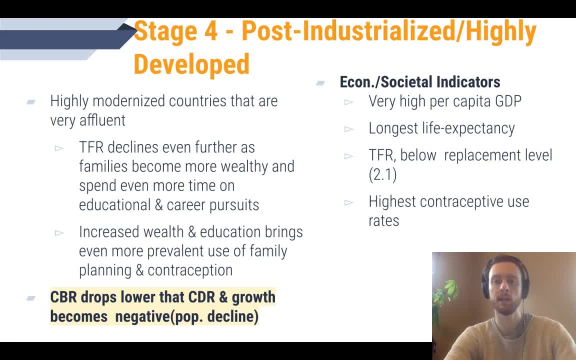 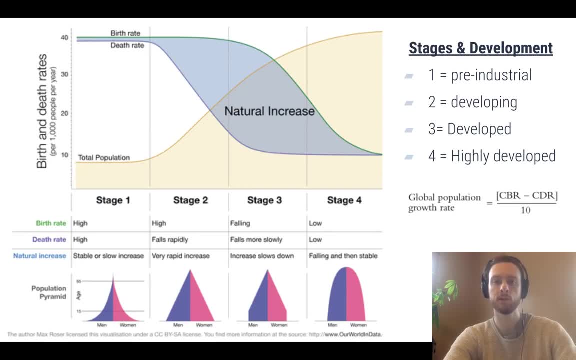 Examples of these countries would include the United Kingdom, Germany, Italy and Japan. Now we'll take a look at this model of demographic transition that can help us kind of visualize How the growth rate changes as a country develops. So if we start out on the left here in phase one, countries have such a high birth rate? 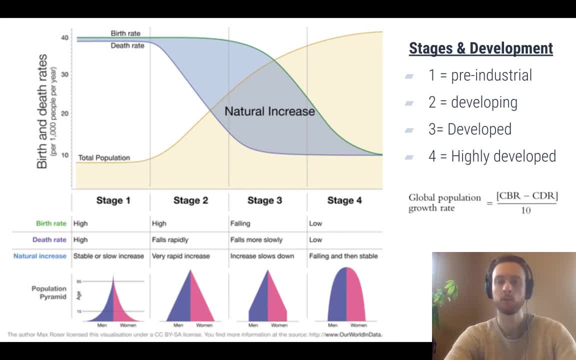 and death rate, that growth is essentially zero And if we were to look at a population age structure diagram, they're going to have a dramatic pyramid that quickly pulls in towards the center, because the death rate is so high that many infants are not even surviving into their reproductive years and many of the 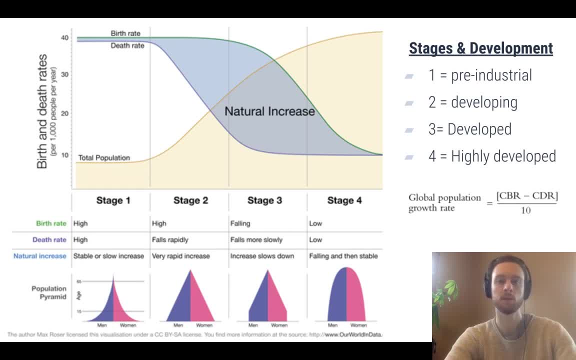 reproductive age. individuals are dying before, Before Post-reproductive age, So this is going to give us growth that is slower, non-existent. Remember, though, that there aren't really any true stage one countries in the world, So even the very poorest nations on earth, have infant mortality rates and death rates. 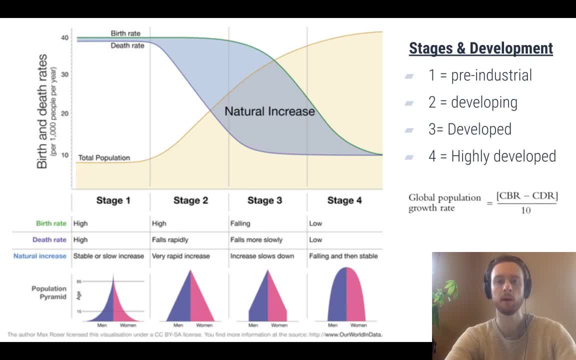 that are lower than their crude birth rates. So we don't see populations that are this underdeveloped. Then we have stage two countries, and these will start to industrialize, which brings clean water, stable food supply and healthcare to much of the country. 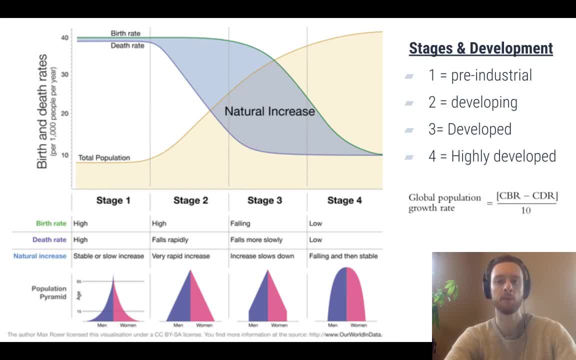 And this causes death rate to fall rapidly. So if we look at the graph here, we'll see that the blue line, the death rate will fall dramatically in stage two, but birth rate stays high. And remember this is for that reason that we discussed, which is kind of the idea of 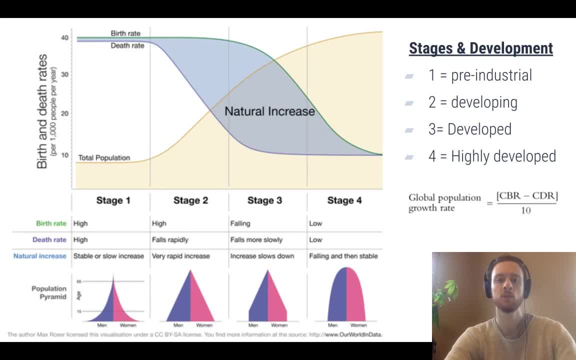 population momentum or generational lag time. So it takes a while for women to get increased educational opportunities and it also takes a while for societal and cultural norms to change To normalize having fewer children. So we maintain a high birth rate all throughout phase two, even though the death rate is declining. 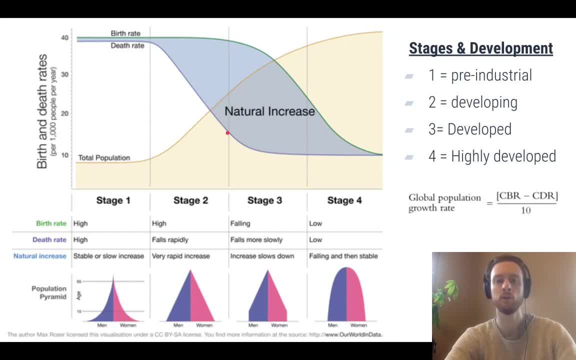 substantially due to increased access to healthcare, food, water And, as a result, we can see our population in the background. This growth rate is rising steadily Now, if we go down and look at the population pyramid, we'll see a pretty nice upward triangle. 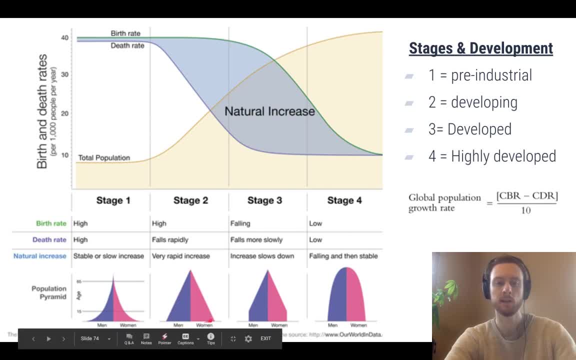 or pyramid here, with our largest group being the pre-reproductive age cohort At the bottom, And that again is going to indicate rapid increase in population, rapid growth. Now, if we look at stage three, the major characteristic of stage three is that we have a low death. 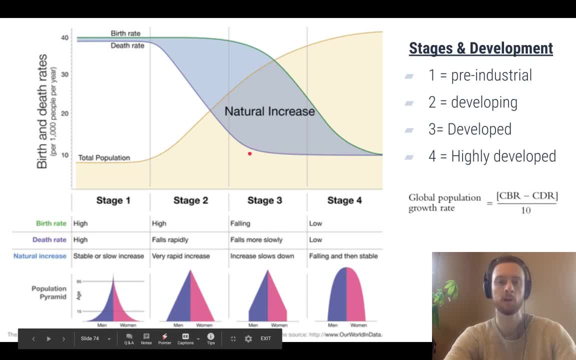 rate because people are getting access to clean water, They're getting access to healthcare and vaccines, But the birth rate starts to fall and that's the real marker of stage three. beginning Birth rate falls as that generational lag catches up. In the beginning it becomes more acceptable for families to have fewer children. 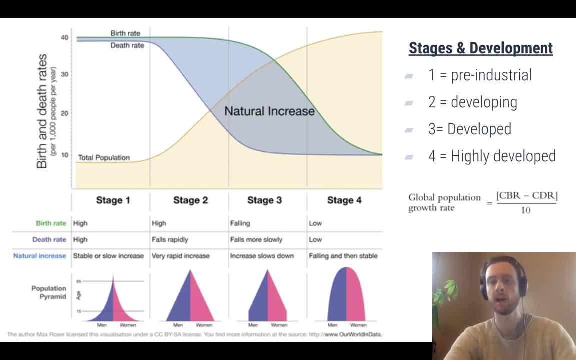 There's a decreased need for children to work on farms to provide agricultural labor. Families are spending more time pursuing educational and career opportunities, so they're having fewer children, They're getting married later, And so all of these factors lead to this dramatic decline in birth rate. 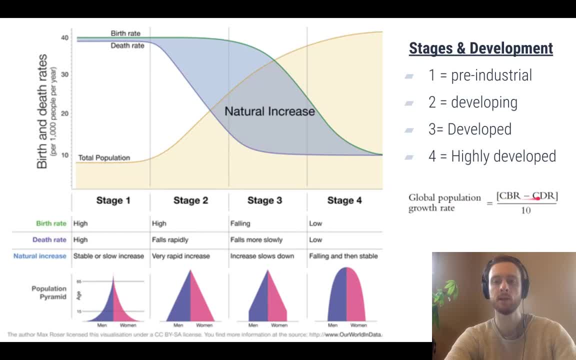 And remember, since growth rate is just equal to CBR minus CDR, if we decrease our birth rate and bring it closer to our death rate, this number gets smaller. So we're going to have a lower growth rate And we can see that reflected by this light orange line here that represents population. 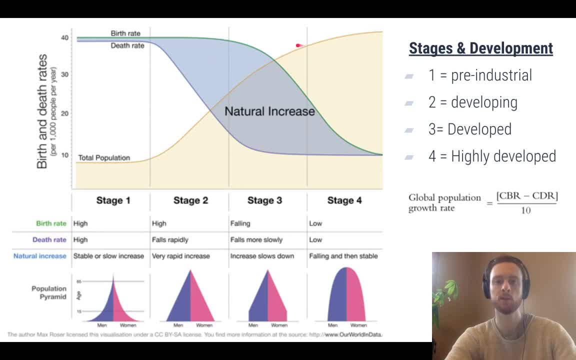 It's still growing, but look what happens to its slope, especially towards the end, It starts to flatten out a little bit. It's getting far less dramatic or less rapid than it was in stage two. Now, if we look at stage four, we're in a very highly developed country. 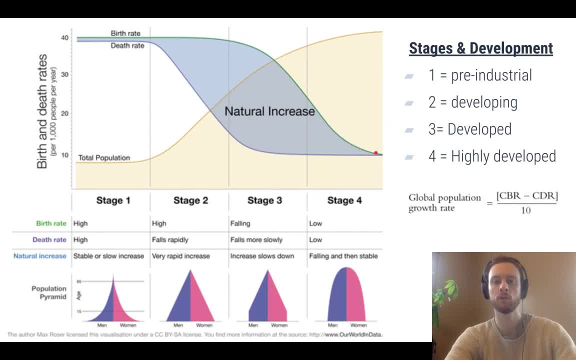 The birth rate continues to fall and it's going to come closer and closer to what we would call replacement lag. So we're going to have a very low birth rate, very low death rate, and so population growth is falling and potentially even declining. if we go later into stage four. 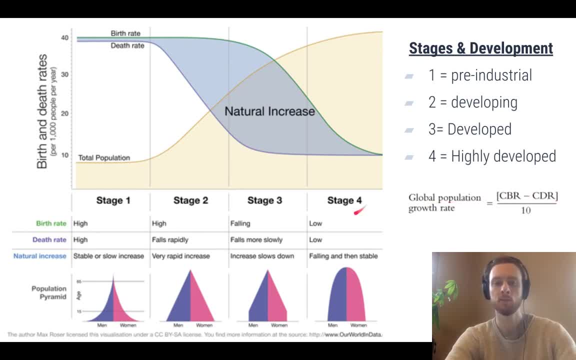 In terms of an age structure diagram, we're going to have a much higher proportion of birth rate and death rate, which is going to bring birth rate and death rate essentially equal. And if we look at our mathematical equation here, if we have birth rate and death rate, 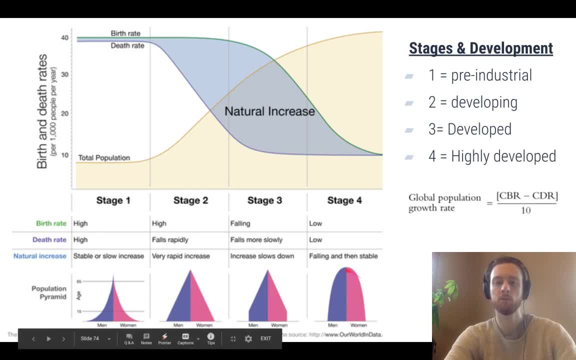 equal. this is going to be a wash, This will be zero And our growth rate will be zero. So we're going to have a much higher proportion of elderly individuals than any of our other stages And in reality, we would actually probably see the pre-reproductive age cohort start. 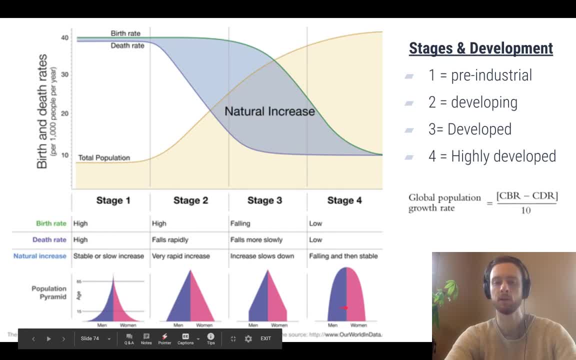 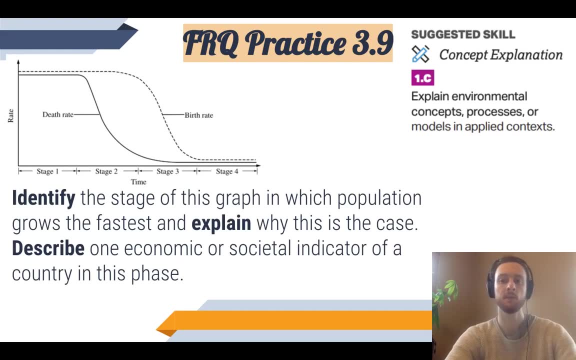 to shrink in and be smaller than our reproductive age cohort. So our FRQ practice today for topic 3.9 is going to involve the science skill of concept explanation, specifically explaining a model in an applied context. So what I want you to do here is see if you can identify the stage of this graph in which 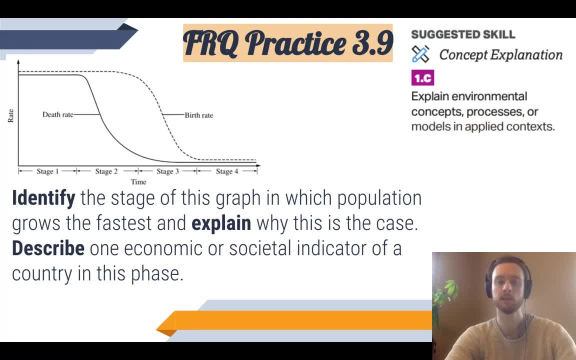 population grows the fastest. Okay, Let's see why this is the case. But then I also want you to think back to those economic and societal indicators of the different stages we talked about and try to describe one indicator of a country that's in this phase.